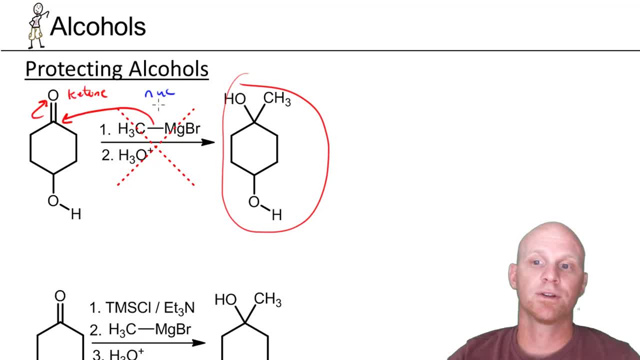 So again, your grignard reagent is a very strong nucleophile, but it's also a very strong base And a bronsted acid base reaction is generally faster than a nucleophile-electrophile reaction. So this grignard reagent, being a nucleophile, looks over at this partially positive carbon and says: 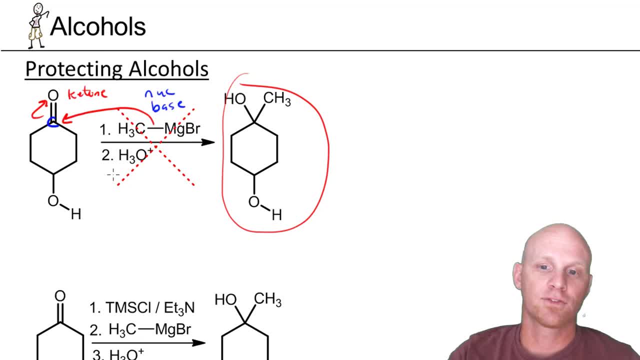 or something akin to that. but then it looks over at this hydrogen right here and says: Oh my goodness, hubba, hubba, you're not supposed to mix me with anything protic. So, and as a result, instead of getting the desired product here, all we did was deprotonate the already existing alcohol. here we'd still have a ketone, we'd end up with an alkoxide ion right here, and then your CH3 just bonds to another H here and becomes CH4, which in this case is a gas- and bubbles out of the solution. 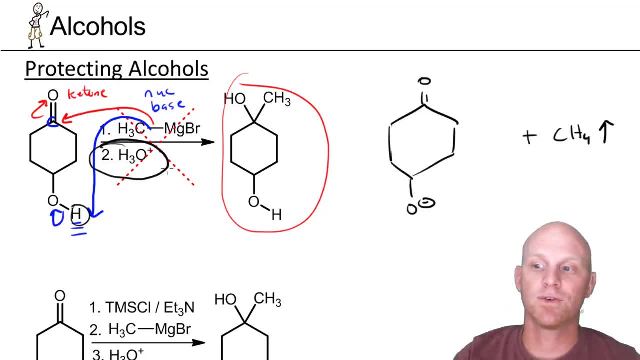 And then when you go to add H3O plus in step two, it just simply reprotonates it and turns it right back- not there, turns it right back into the original reactant. So your grignard reagent is a very strong nucleophile. 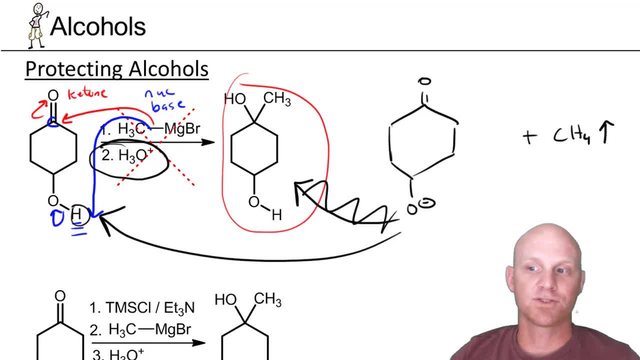 So your grignard reagent is destroyed, converted into methane and your original reactant gets returned back to its original state. You did not accomplish the reaction you wanted to do, So that's why you got the big red X here going through here. 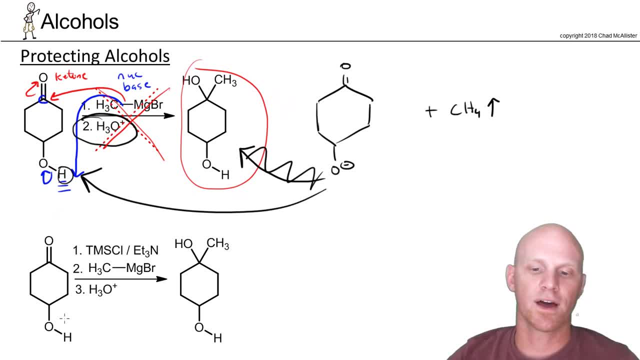 So if you actually want to pull this off, there's a bit more to it and you got to do what we say: protect the alcohol first. So- and I like to think it's really more protecting the grignard reagent from the alcohol, but that's not the way we word it. 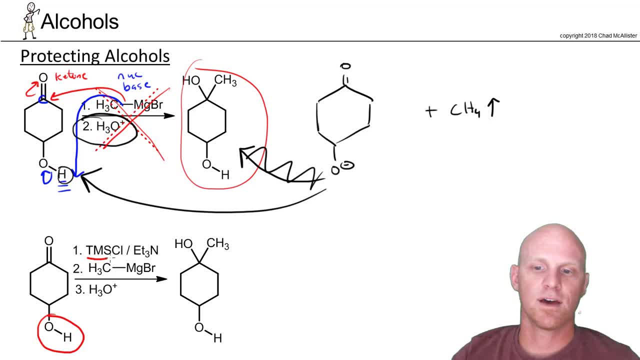 We say we're protecting the alcohol and we protect that here with TMS, TMSCl and triethylamine. we'll talk about what those look like in a little bit here, and once we protect it, we can do our reaction. and then we have to de-protect and we're going to take a little more specific look at what that looks like, as well as what some of these reagents look like as well. 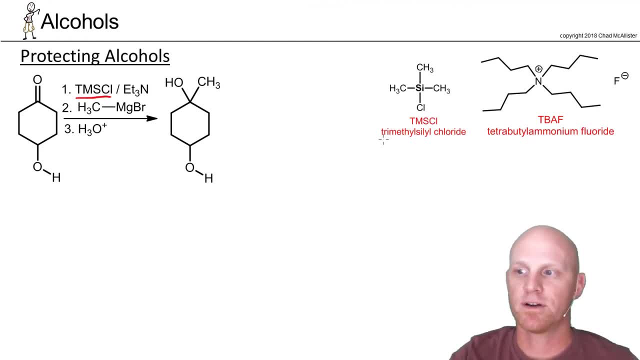 So first of all these reagents, so TMSCl here is trimethylsilyl chloride, so you got a silicon in there. that's the silyl part. so instead of being carbon, it's silicon in the middle there. 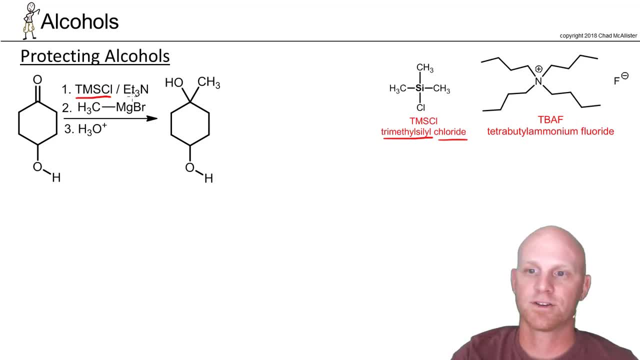 And in this case you've also got triethylamine, which is just simply nitrogen bonded to three ethyl groups. so it needs a pretty decent organic base, and that's what we're dealing with in terms of the protection here. And essentially what's going to happen here is our alcohol is going to come in and attack the silicon atom and kick off the chlorine, so a substitution reaction, and if you kind of look at what that's going to end up looking like here, 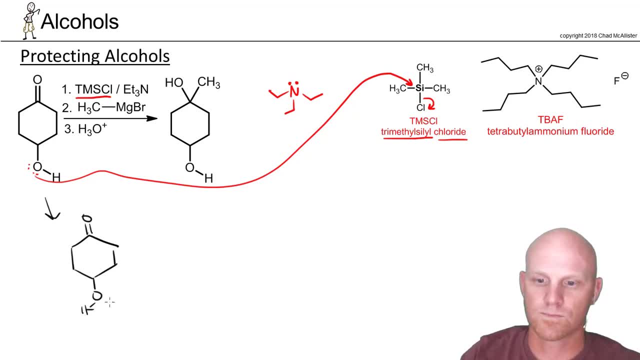 So it's still bonded to the hydrogen. there the oxygen's going to have a positive formal charge and that silicon is still bonded to three methyl groups. so instead of writing CH3s, I'm going to get a little lazy here and write methyl groups. 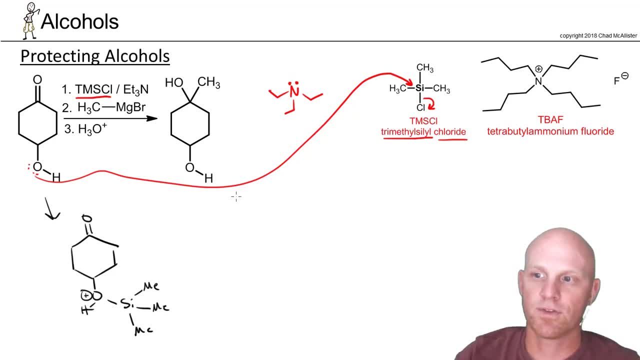 So and then it's the base's job to come and pull that H off. so that's where our triethylamine comes in and deprotonates And now we no longer have an OH. so our solution in this case, this molecule is not protic anymore and I don't have a problem with it actually protonating a grignard reagent and destroying a grignard reagent. 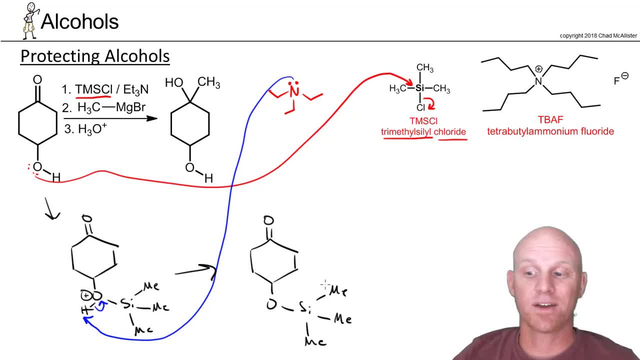 The alcohol is now protected, and what's nice is I can remove this back off with either H3O+ or some fluoride ions, Which we have a special way of getting in there, if we choose to do it that way. In our case, we're just going to use H3O+ at the end of this reaction. it'll serve a two-fold purpose. 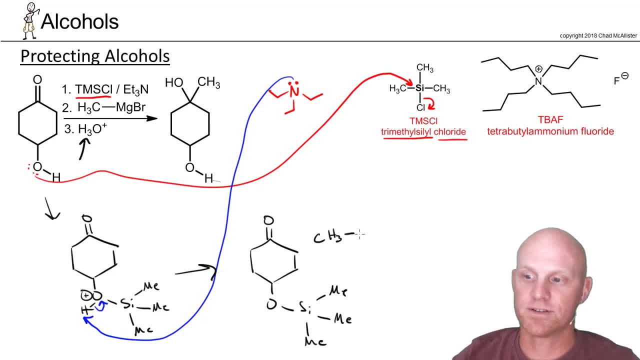 But the big thing is that now I can add my grignard reagent so and it's free to attack my ketone, because there's no alcohol for it to react with in an acid-base reaction. So that's going to get us to an alkoxide ion with the methyl group attached. 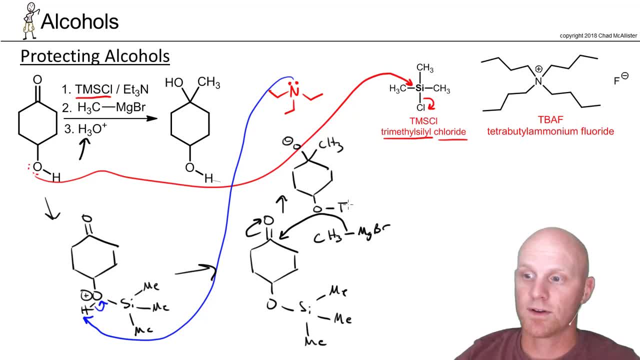 One thing, by the way, we often abbreviate this as OTMS in this case. and finally, we'll finish this reaction off by adding H3O+, and that H3O+ is going to accomplish two things. So one, it's going to protonate this oxygen, turning it into an OH, but also it's going to deprotect, turning that back into an alcohol as well.